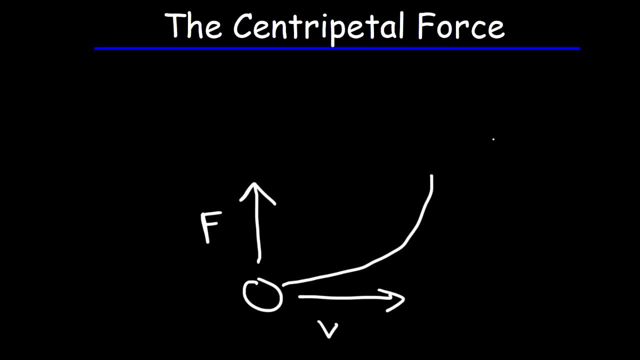 It causes an object to turn in a circle. Now, centripetal has the keyword centri or center-seeking. This is a center-seeking force, And so the force is always directed. It's always directed towards the center of the circle. 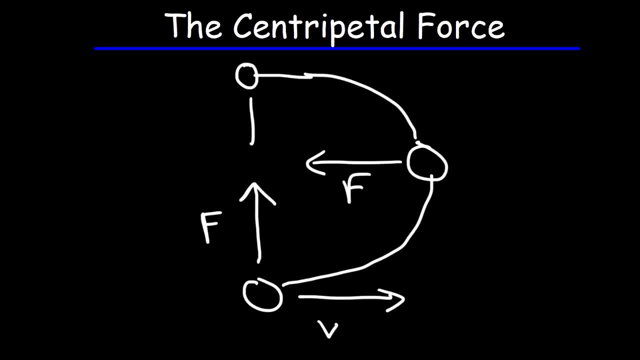 And thus that is a centripetal force. It's any force that keeps an object moving in a circle. Now, the centripetal force is not a force by itself. In fact, it's caused by other forces. So here's an example. 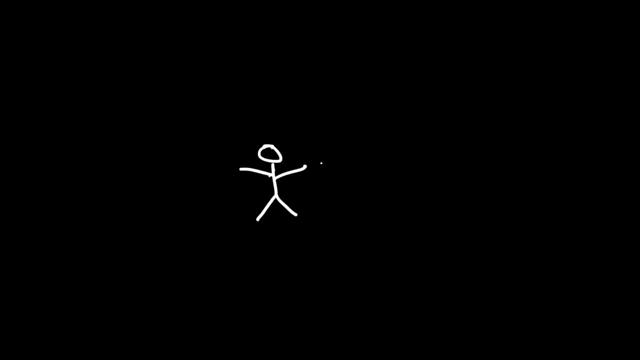 Let's say, if we have a person and he has a ball attached to a rock and he's swinging his ball in a circle, So what force provides the centripetal force in this case? Anytime you have a force acting through a rope? 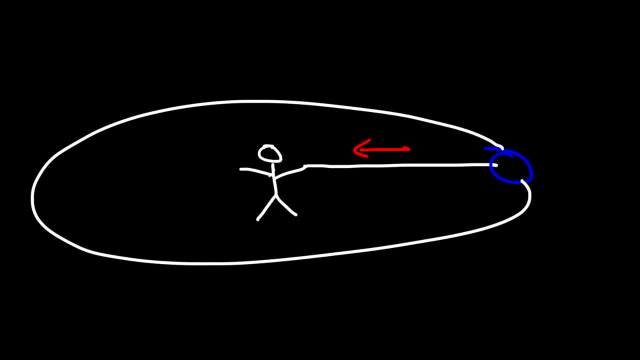 what is that force called? This force is the tension force. So in this particular situation, tension provides the centripetal force. It keeps the ball moving in a circle. Now let me give you another situation. Let's say, if you have a car, 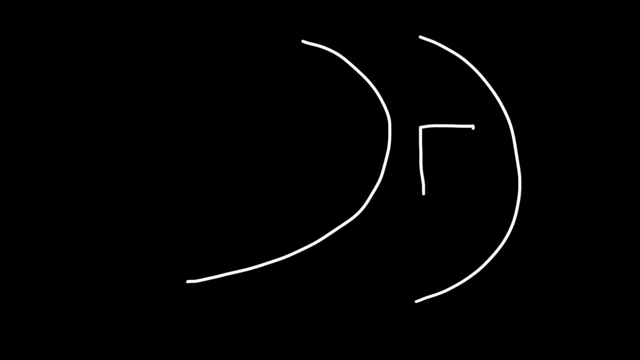 which I'm just going to draw a box. but this is a car and it's turning on a road. It's following the curvature of a road and it's turning. The fact that it's turning, there's some force that it's causing it to turn. 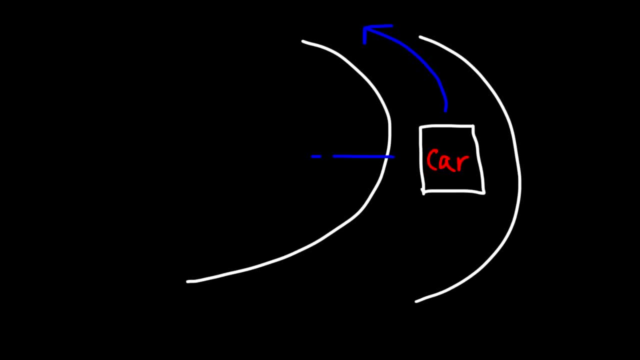 Let's say, if it's moving at constant speed and turn at the same time, So the fact that it's turning, there's some force that it's causing it to turn. Let's say, if it's moving at constant speed and turn at the same time. 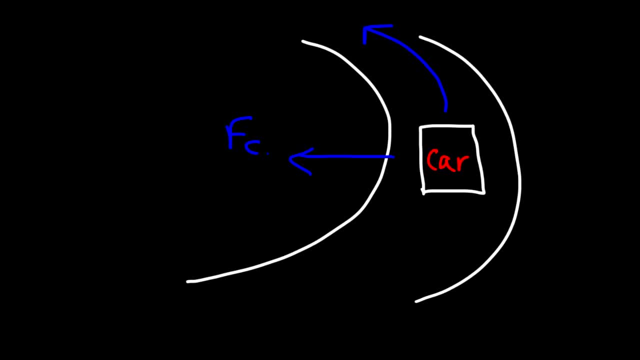 So there is a centripetal force acting on this car because it's moving in a circular path. What centripetal force, or rather, what other force, provides the centripetal force in this case, If you see a situation like this? 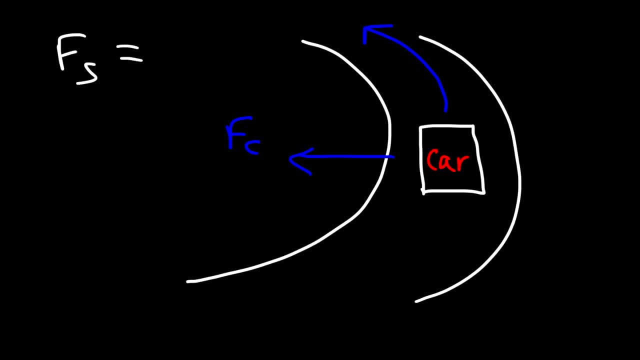 static friction provides the centripetal force. So if you're dealing with a physics problem that has a car turning on a road like this, make sure you set static friction equal to a centripetal force. Now the formula for static friction is mu s times the normal force. 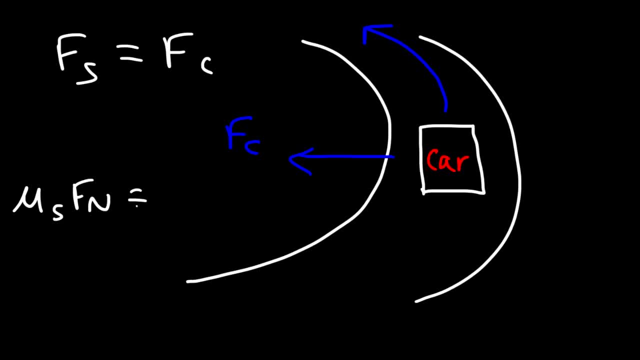 It's less than or equal to this quantity, And for the centripetal force it's mv squared over r. The normal force on a flat surface is simply mg, So in this case we could cancel m in the expression. So for a word problem that involves a car. 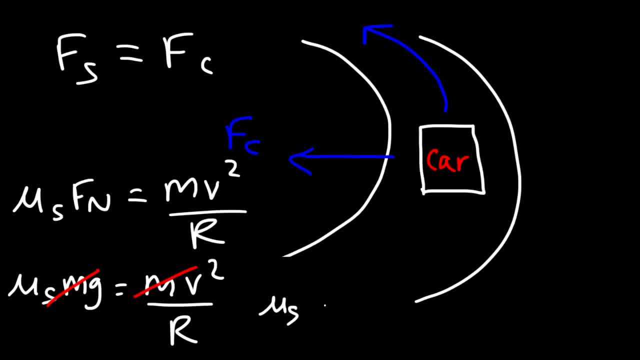 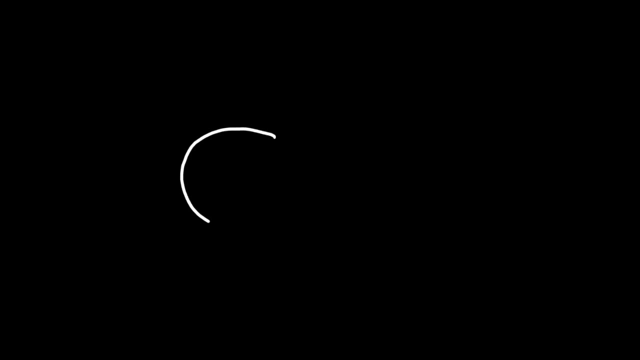 turning on a road. you have this expression: The coefficient of static friction times the gravitational acceleration is equal to v squared over r, And I'm going to post some links in which you can practice these problems in another video. Now let's say this is the sun. 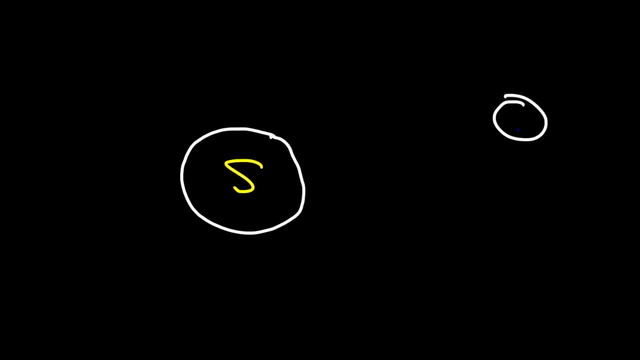 and here we have the earth, And the earth is orbiting the sun, So the earth is moving in a nearly circular path around the sun, Which means that there's a force that's acting as a centripetal force, in this case, to keep the earth moving. 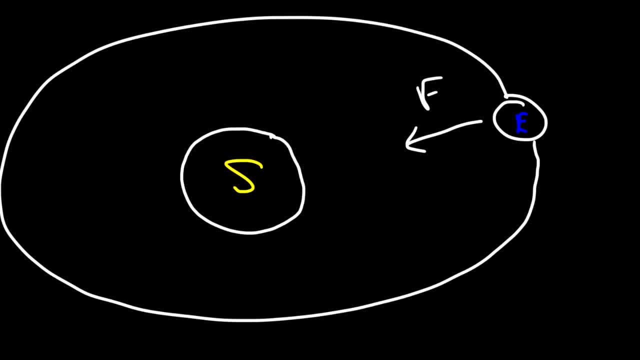 with uniform circular motion. What force provides the centripetal force? in this case, The force that keeps the earth in orbit around the sun is the gravitational force, And so gravity provides the centripetal force in this example. Without gravity, the earth will fly off in a tangent. 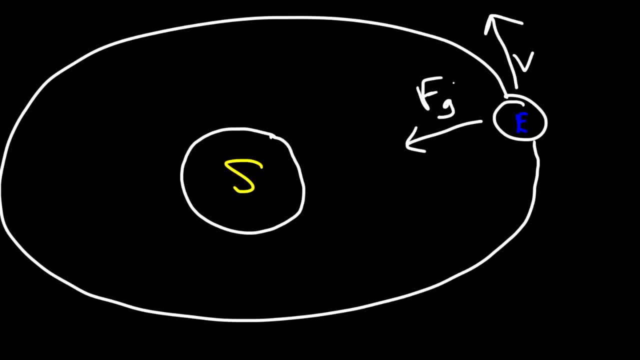 away from the sun deep into outer space. But because we have these two forces that are perpendicular to each other, the earth instead turns in a circular path, And so make sure you understand this Anytime you have a force that's perpendicular to the velocity component. 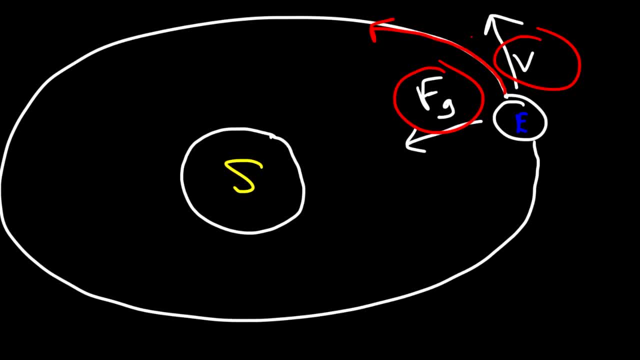 I mean the velocity vector. the force doesn't speed up or slow down the object. It has no effect on the speed If it's perpendicular to the velocity of the object. the force can only change its direction. Now let's focus on the equation. 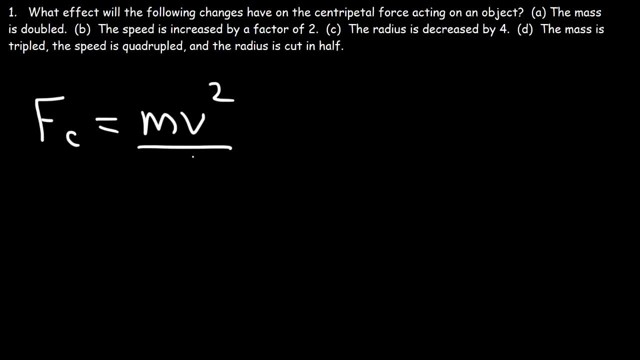 that relates to the centripetal force acting on the object. It's mv squared over r. So here's a question for you: If the mass of the object increases, what will happen to the centripetal force? Will it increase or decrease? 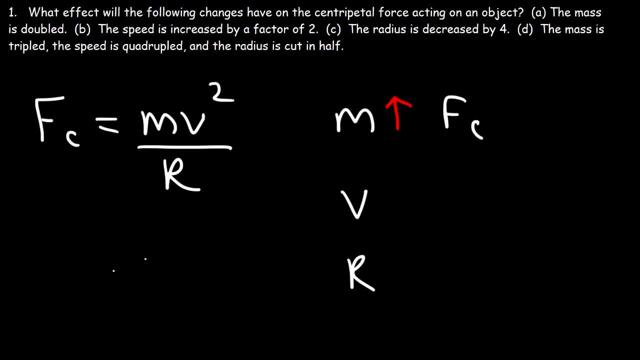 Because the mass is in the numerator of the fraction. increase in the mass will increase the centripetal force. The same is true for the velocity. If you increase the speed of the object, the centripetal force that's needed to keep the object moving in a circle. 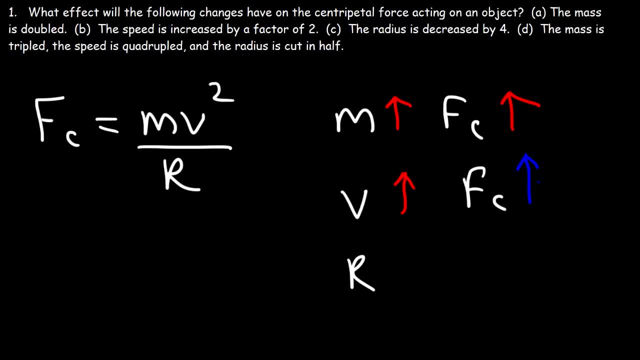 must be increased as well, Otherwise the object is going to fly out of the circle. So the greater the speed, the more centripetal force that is needed to keep the object moving in a circle. Now what about if we increase the radius? 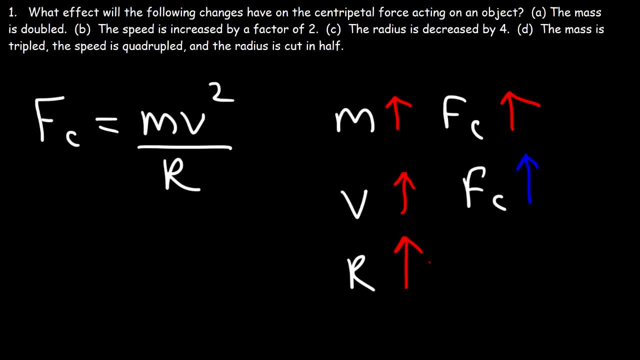 of the circle. What's going to happen to the centripetal force that is needed to keep the object moving in a circle? If you use a wider circle, the centripetal force that's needed to keep it in that circle will decrease, because r is in the denominator of the. 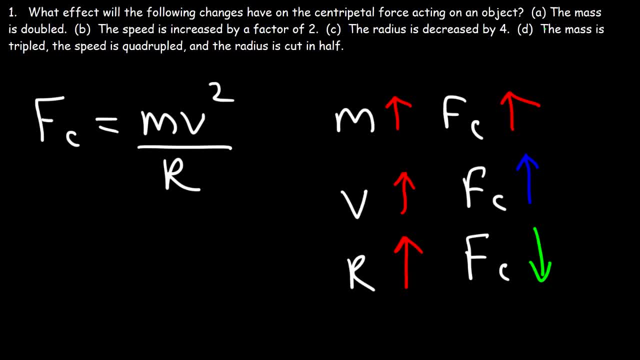 fraction, And so let's focus on questions like these. What effect will the following changes have on the centripetal force acting on an object? What's going to happen if we double the mass? We know the centripetal force will increase. 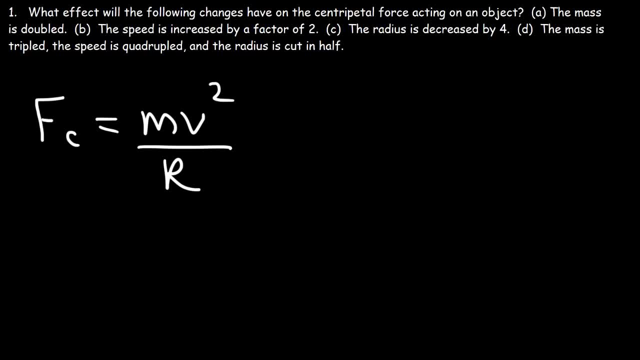 but by what factor? Now, the way in which you can get the answer is as follows: Everything that doesn't change, replace it with a 1.. Now, because the mass increased by the factor of 2, replace m with 2.. 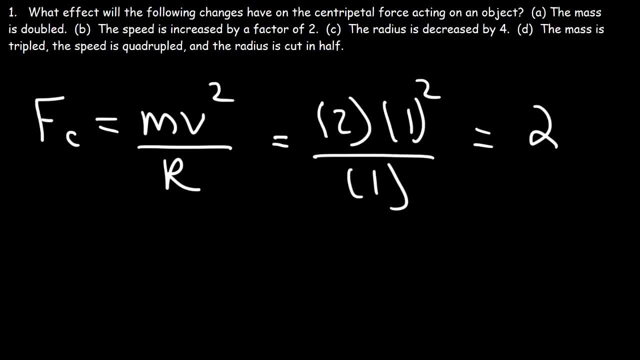 v and r we're going to replace with 1.. So we get a value of 2.. This tells us that the centripetal force will double if we double the mass. Now let's move on to part b. So what effect will it have? 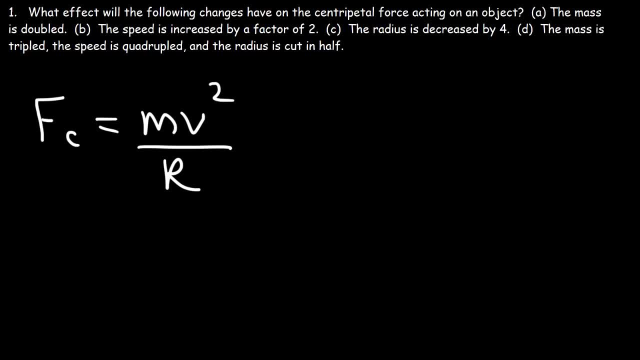 on the centripetal force if the speed is increased by a factor of 2?? So the mass and the radius doesn't change, so we're going to replace it with a 1.. But the speed is doubled, so we're going to replace it with a 2.. 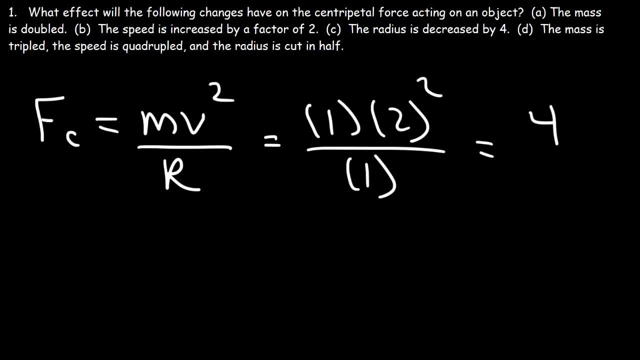 2 squared is 4, and so this tells us that the centripetal force will increase by a factor of 4.. Now what about part c? The radius is decreased by 4.. Let's say, decreased by a factor of 4.. 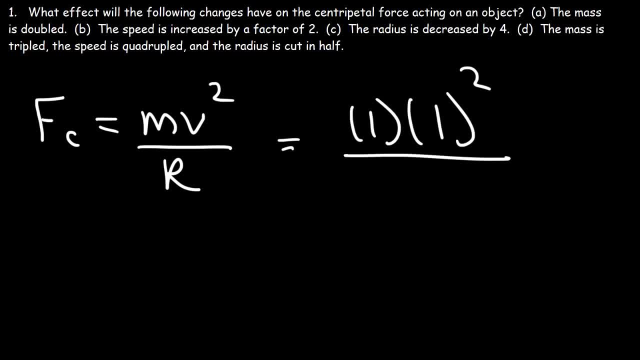 So what should we do? m and v doesn't change, so we're going to replace that with a 1.. If the radius is decreased by a factor of 4, that means that it's 1 fourth of its original value. So we have: 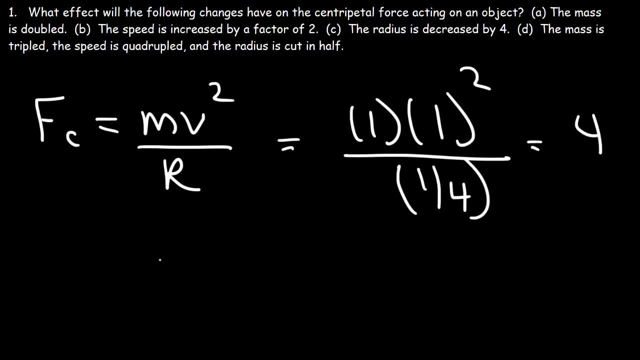 1 divided by 1, fourth, which is 4.. If you want to show your work with that, what you need to do is multiply the top and the bottom by 4.. 4 times 1, fourth is 1, and so you get 4.. 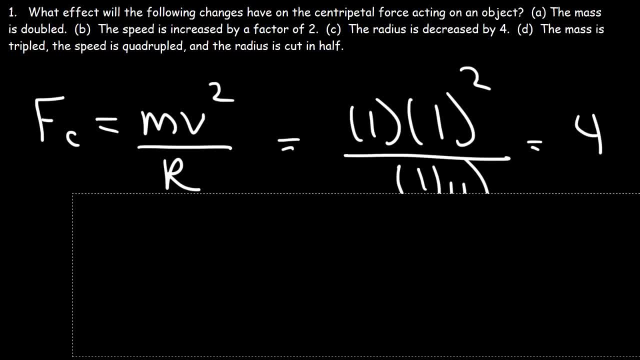 Now what about the last one, Part d? What effect will tripling the mass, quadrupling the speed and cutting the radius in half have on the centripetal force acting on the object? So all we got to do is plug in these numbers. 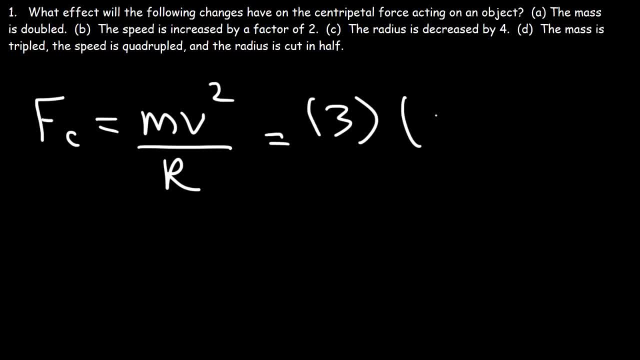 So we're going to triple the mass, replace it with a 3.. The speed is quadrupled, so we're going to replace that with a 4. and the radius was cut in half. so let's replace r with 1 half, So we have. 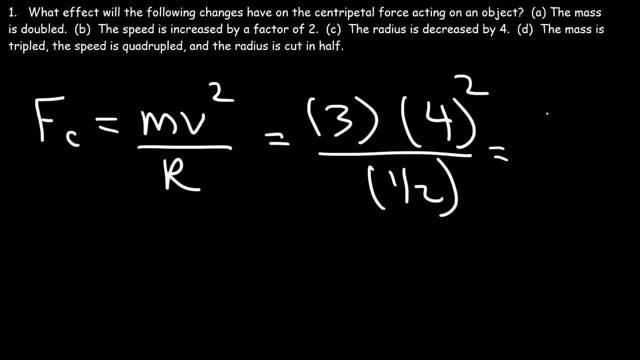 4 squared, which is 16.. 16 times 3 is 48, and 48 divided by a half is the same as 48 times 2, and so we get 96. So the centripetal force will increase by a factor of 96 in this case. 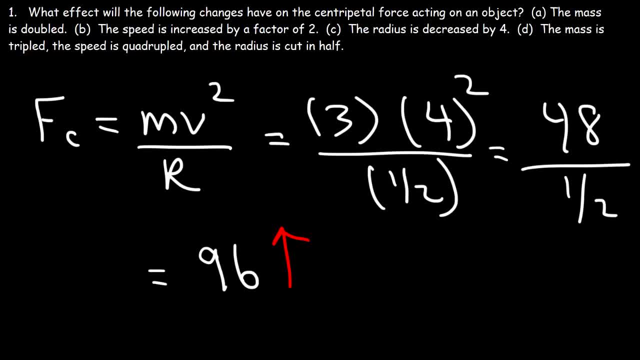 And that's basically it for this video. So I want to give you a simple introduction into centripetal force. Now, for those of you who want actual harder problems regarding this topic, check out the links in the description section, Because I'm going to post some. 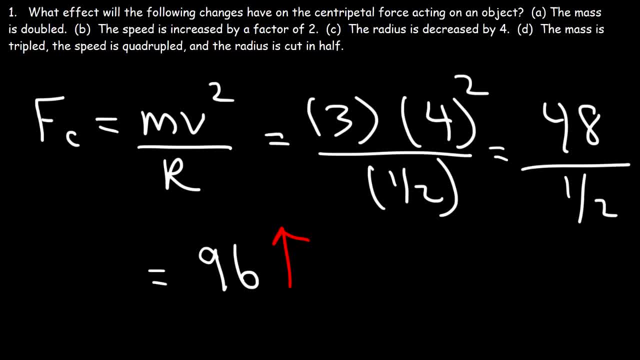 links to other videos that have more problems on this topic And other videos that you might be interested into. And, when you get a chance, check out my new physics video playlist, because I have these topics listed in order And if you like this video, don't forget.